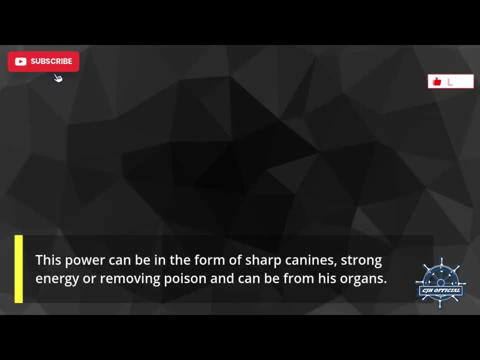 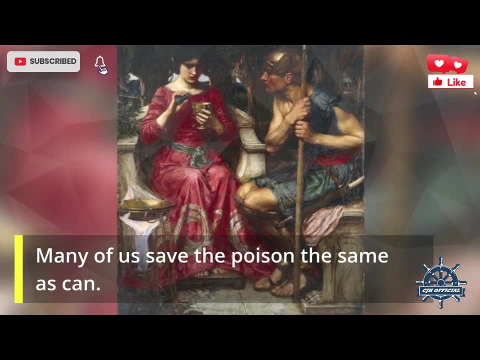 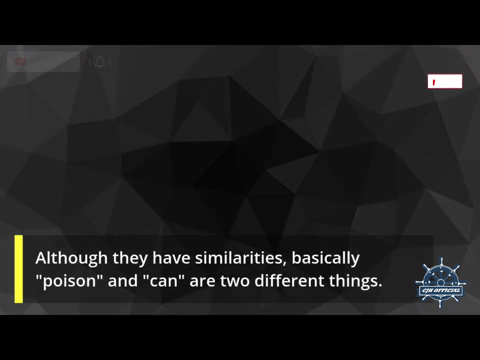 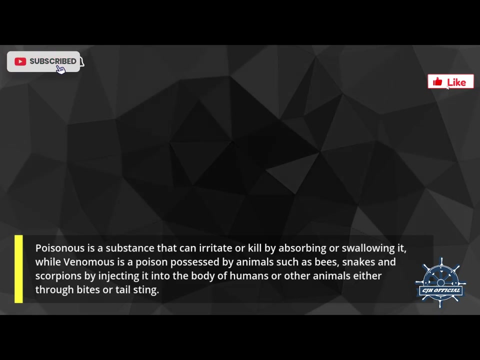 This power can be in the form of sharp canines, strong energy or removing poison, and can be from his organs. Many of us save the poison, the same as Ken. Although they have similarities. basically, poison and can are two different things. Poisonous is a substance that can irritate or kill by absorbing or swallowing it, while venomous is a poison possessed by animals such as bees, snakes and scorpions by injecting it into the body of humans or other animals, either through bites or tail sting. Poisonous is a substance that can irritate or kill by absorbing or swallowing it, while venomous is a poison possessed by animals such as bees, snakes and scorpions by injecting it into the body of humans or other animals, either through bites or tail sting. Poisonous is a substance that can irritate or kill by absorbing or swallowing it, while venomous is a poison possessed by animals such as bees, snakes and scorpions by injecting it into the body of humans or other animals, either through bites or tail sting. 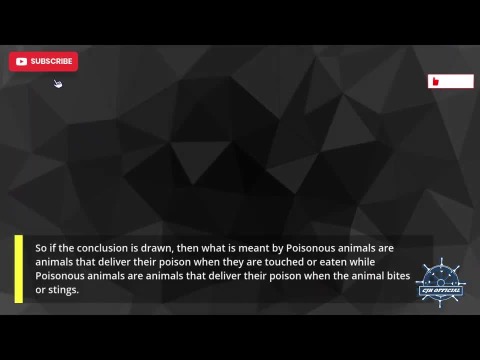 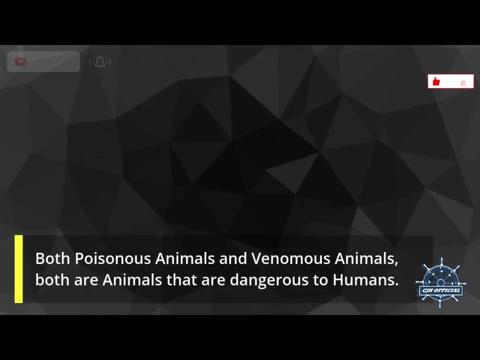 So, if the conclusion is drawn, then what is meant by poisonous animals are animals that deliver their poison when they are touched or eaten, while poisonous animals are animals that deliver their poison when the animal bites or stings. Both poisonous animals and venomous animals: both are animals that are dangerous to humans. 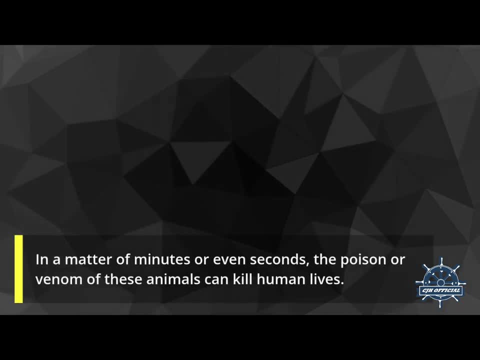 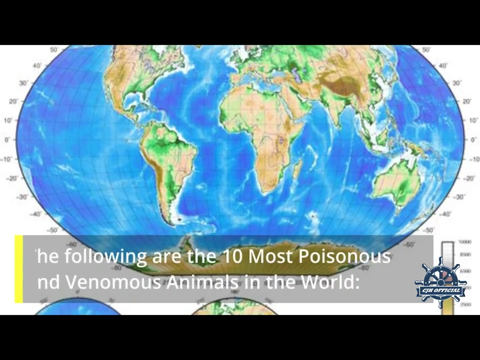 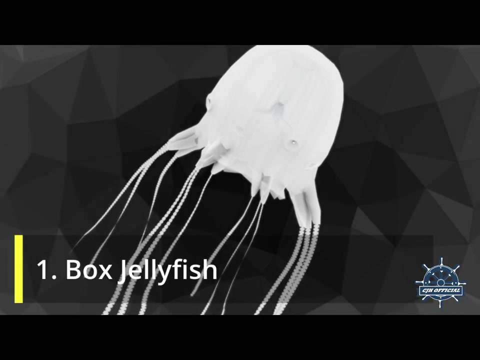 In a matter of minutes or even seconds. the poison or venom of these animals can kill human lives. Therefore, we need to be careful when we meet these animals. The following are the 10 most poisonous and venomous animals in the world: 1. Box Jellyfish. 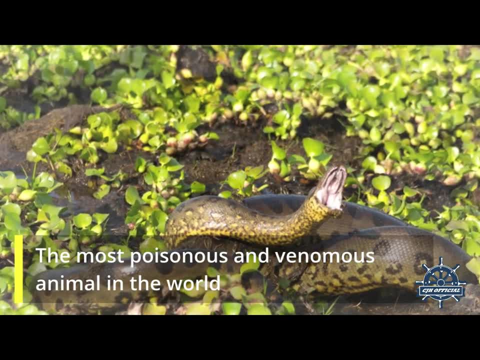 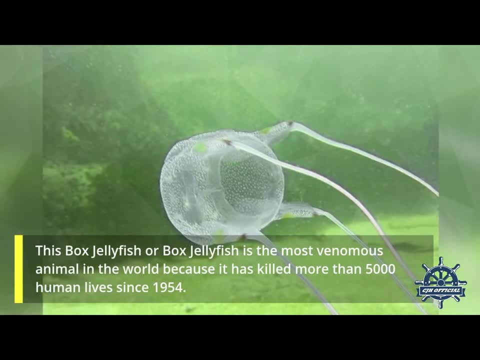 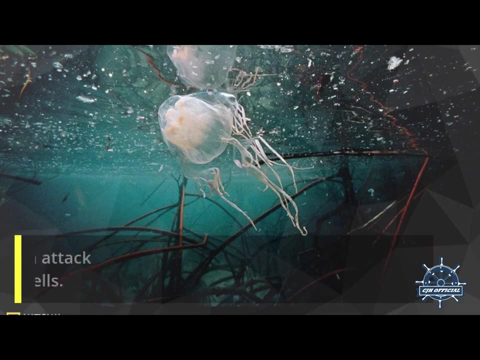 The most poisonous and venomous animal in the world. This box jellyfish, or box jellyfish, is the most venomous animal in the world because it has killed more than 5,000 human lives since 1954.. The poison from this box jellyfish can attack the heart, nervous system and skin cells. 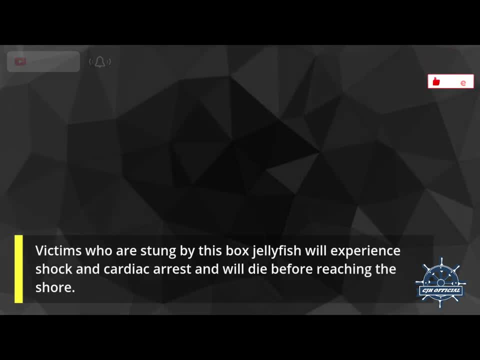 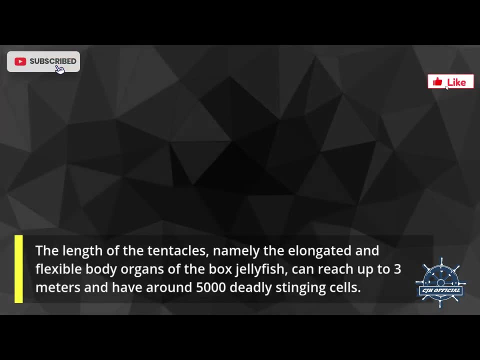 Victims who are stung by this box jellyfish will experience shock, The shock and cardiac arrest and will die before reaching the shore. The length of the tentacles, namely the elongated and flexible body organs of the box jellyfish, can reach up to 3 meters and have around 5,000 deadly stinging cells. 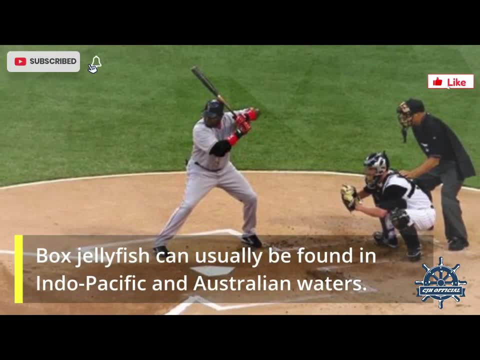 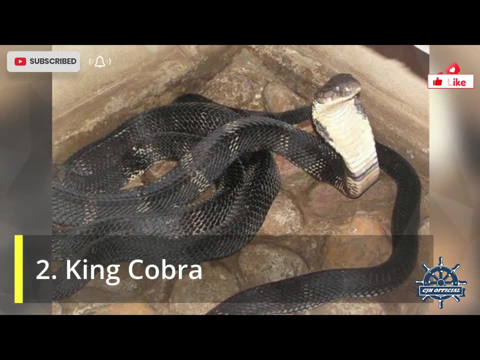 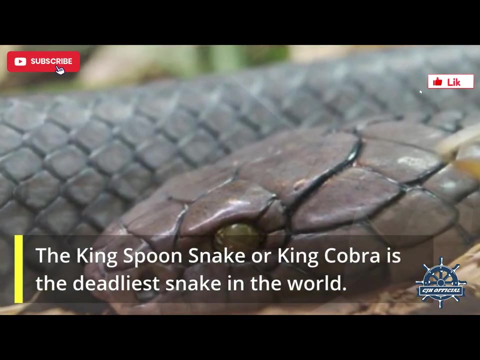 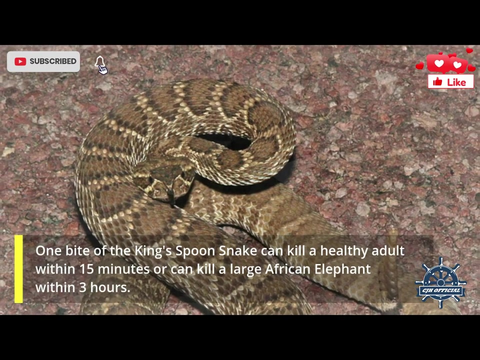 Box jellyfish can usually be found in Indo-Pacific and Australian waters. 2. King Cobra, The king spoon snake, or king cobra, is the deadliest snake in the world. One bite of the king spoon snake can kill a healthy adult within 15 minutes, or can kill a large African elephant within 3 hours. 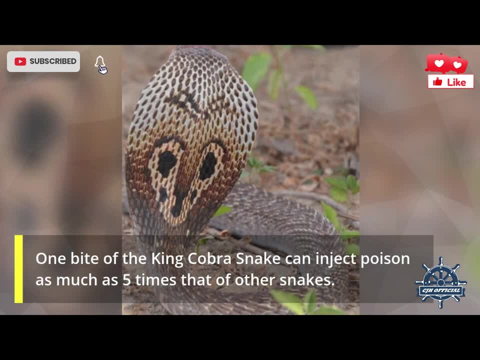 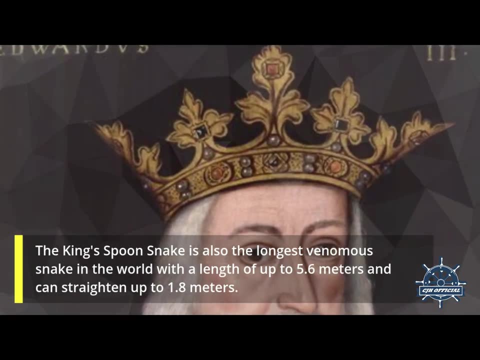 One bite of the king cobra snake can inject poison as much as five times that of other snakes. 3. King Spoon Snake. The king spoon snake is also the largest snake in the world, longest venomous snake in the world, with a length of up to 5.6 meters, and can 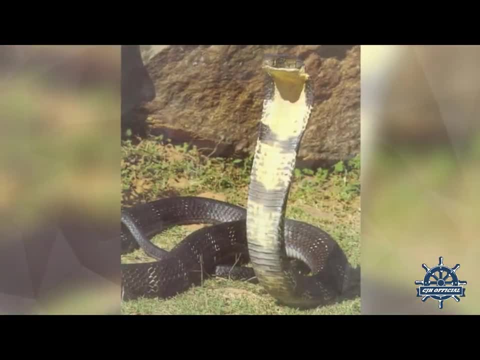 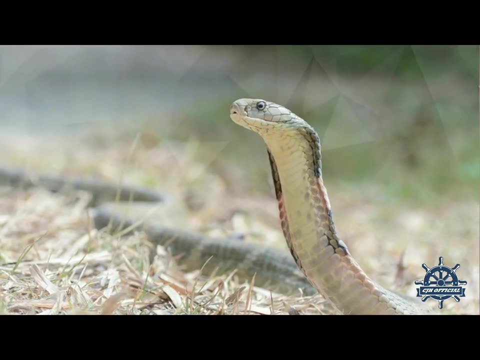 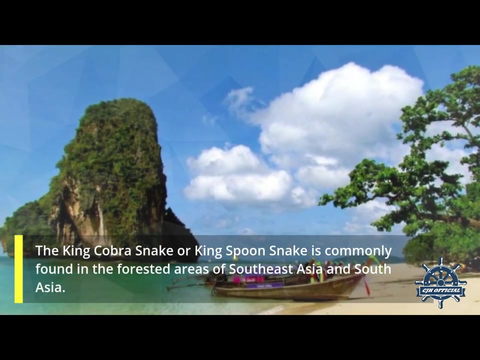 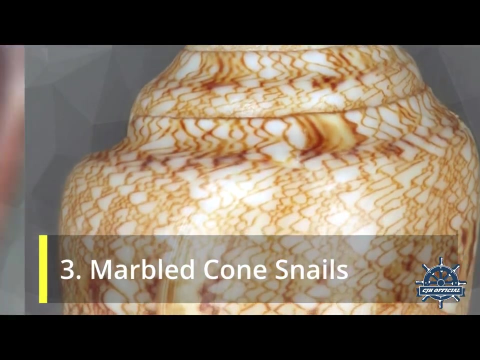 straighten up to 1.8 meters, said the king, because the king cobra snake also preys on other types of snakes. the king cobra snake, or king spoon snake, is commonly found in the forested areas of southeast asia and south asia. three marbled cone snails. 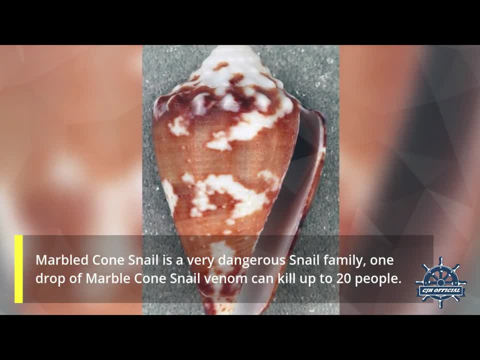 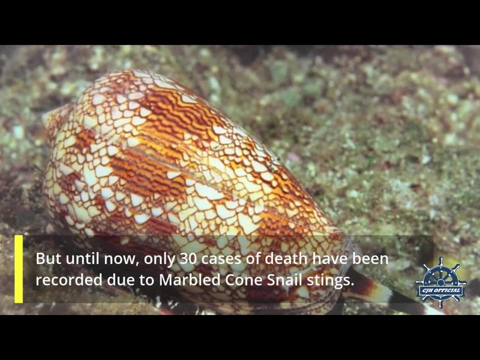 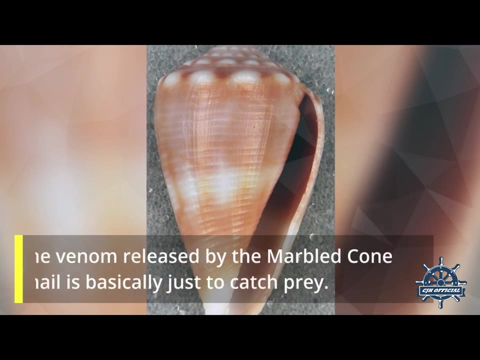 marbled cone snail is a very dangerous snail family. one drop of marble cone snail venom can kill up to 20 people, but until now only 30 cases of death have been recorded due to marbled cone snail stings. the venom released by the marbled cone snail is basically just to catch prey. 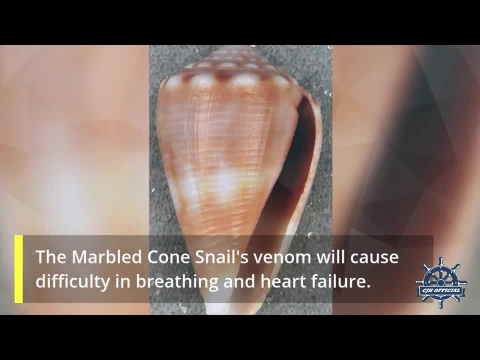 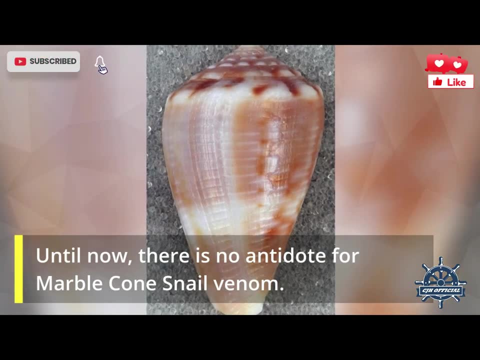 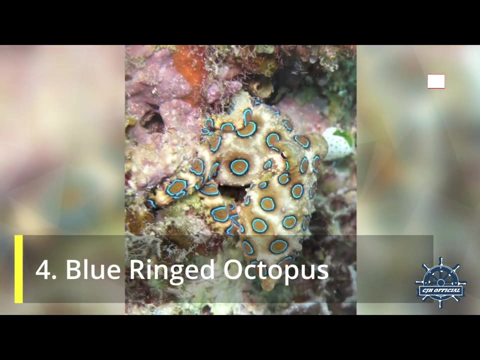 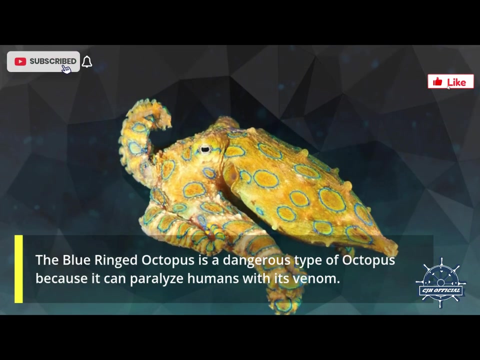 the marbled cone snail's venom will cause difficulty in breathing and heart failure. until now, there is no antidote for marble cone snail venom. 4. blue-ringed octopus. the blue-ringed octopus is a dangerous type of octopus because it can paralyze. 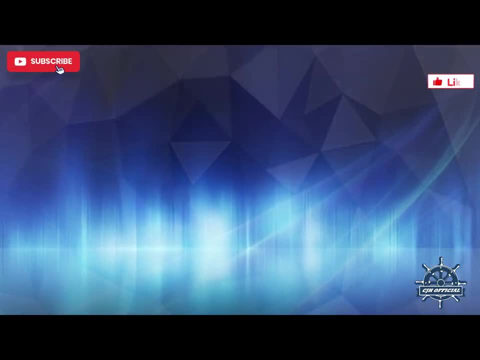 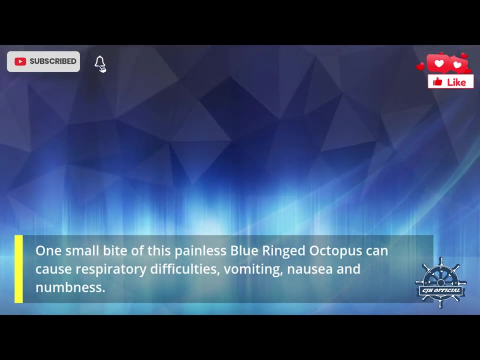 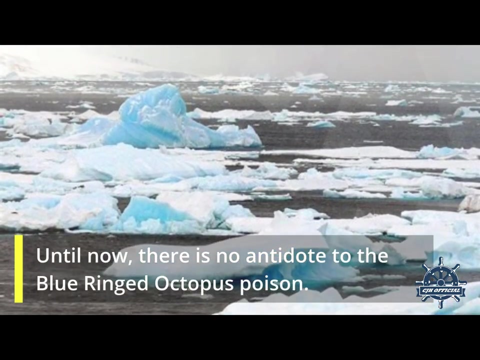 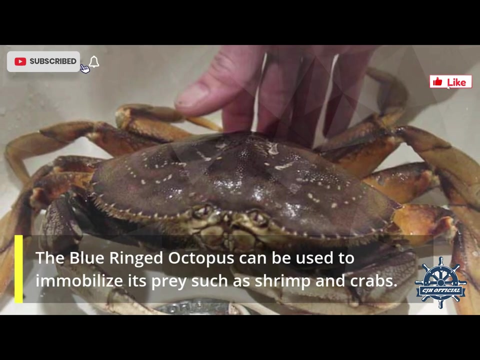 humans with its venom. one small bite of this painless blue-ringed octopus can cause respiratory difficulties, vomiting, nausea and numbness. until now, there is no antidote to the blue-ringed octopus poison. the blue-ringed octopus can be used to immobilize its prey, such as shrimp and 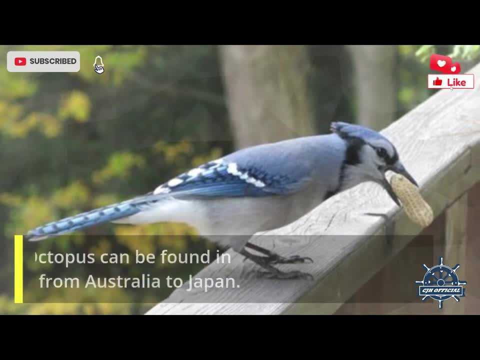 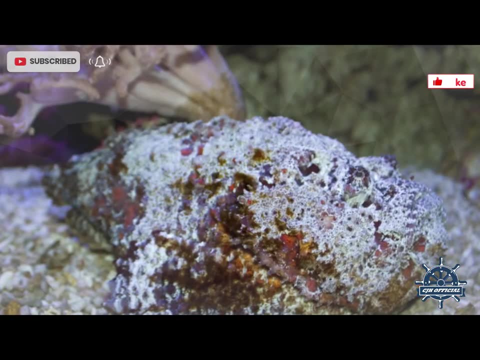 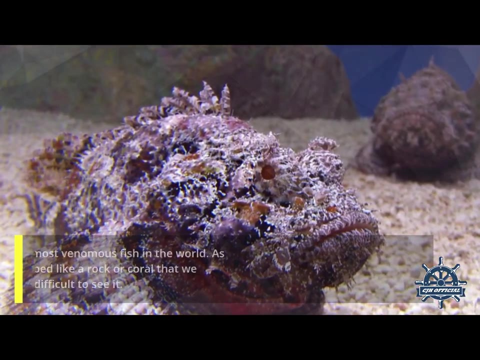 crabs. the blue-ringed octopus can be found in the pacific ocean from australia and the australia to japan. the blue-ringed octopus can be found in the pacific ocean from australia to japan. 5. stonefish: the stonefish, or stonefish, is the most venomous fish in the world. 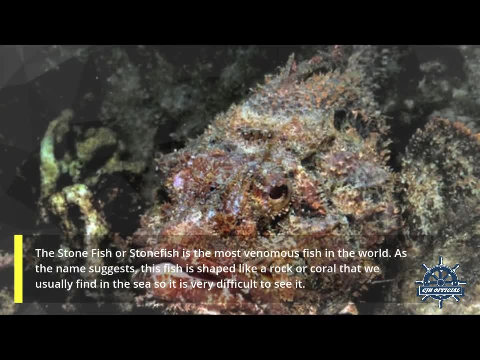 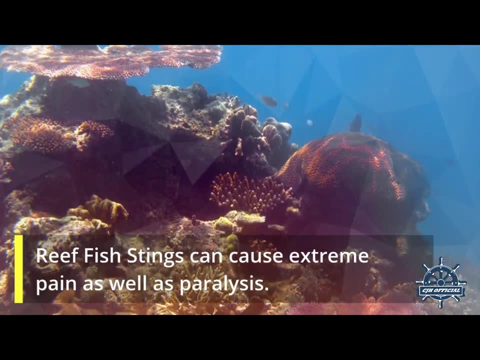 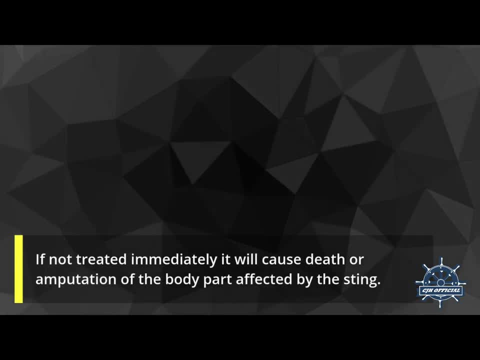 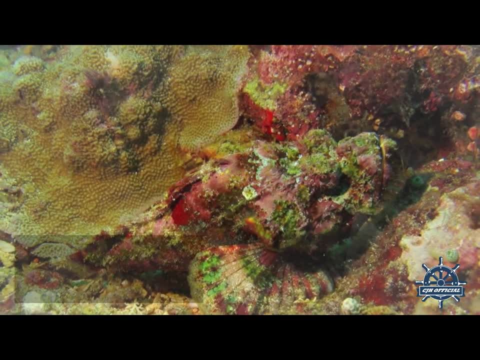 if not treated immediately, it will cause death or amputation of the body part affected by the sting. stonefish, also known as coral fish, are found in stonefish. also known as coral fish are found in stonefish. also known as coral fish are found in the tropical waters of the pacific ocean and. 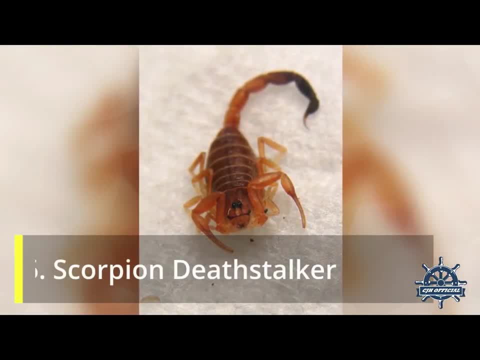 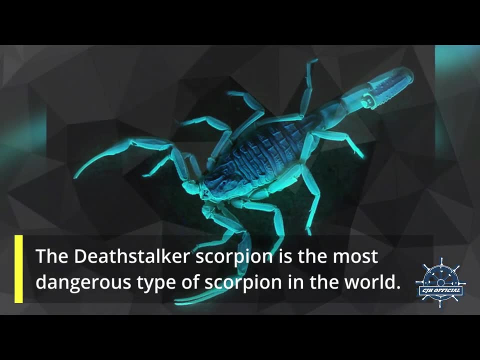 the tropical waters of the pacific ocean and the tropical waters of the pacific ocean and the indian ocean. 6. scorpion- death stalker. the death stalker scorpion is the most the death stalker scorpion is the most. the death stalker scorpion is the most dangerous type of scorpion in the world. 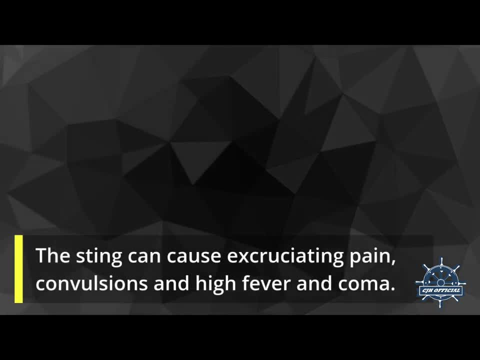 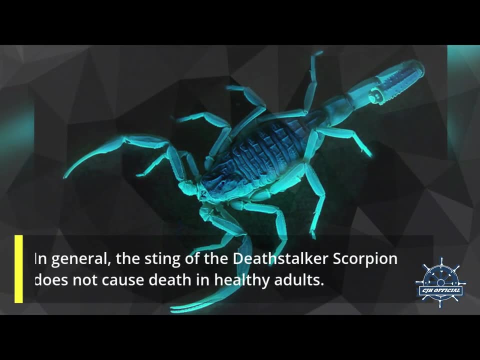 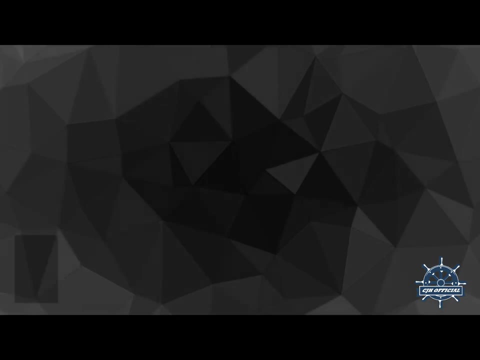 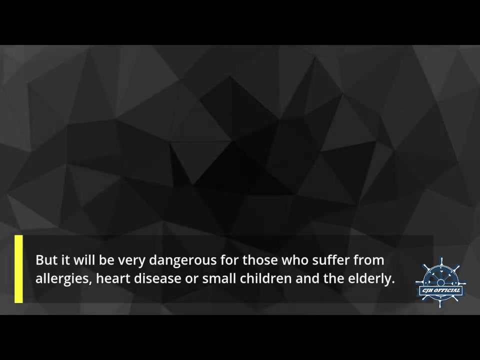 dangerous type of scorpion in the world. The sting can cause excruciating pain, convulsions and high fever and coma. In general, the sting of the death stalk or scorpion does not cause death in healthy adults, But it will be very dangerous for those who suffer from allergies, heart disease or small children and the elderly. 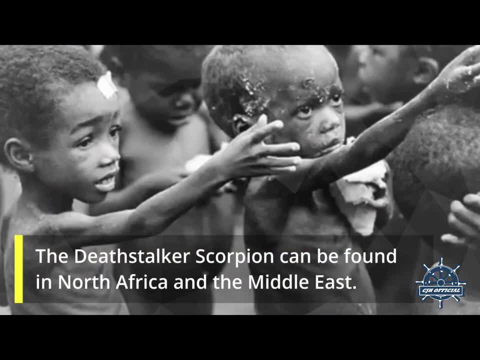 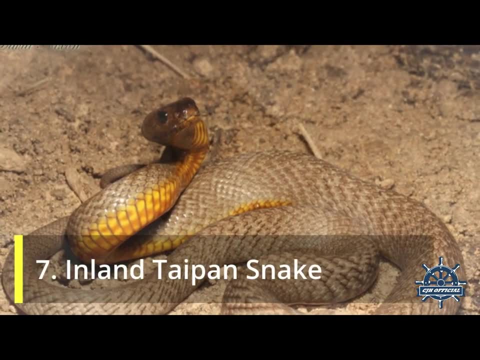 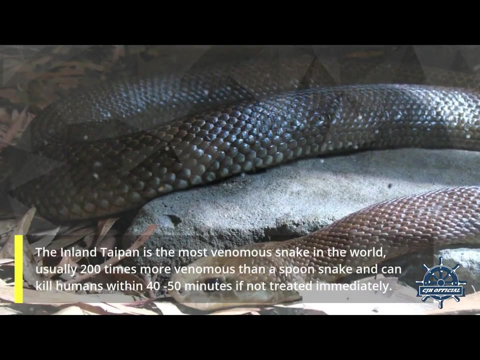 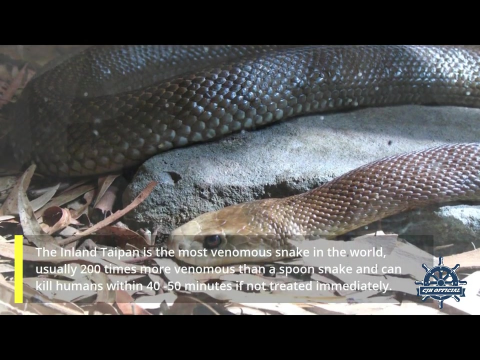 The death stalk or scorpion can be found in North Africa and the Middle East. 7. Inland Taipan Snake. The Inland Taipan is the most venomous snake in the world, usually 200 times more venomous than a spoon snake and can kill humans within 40-50 minutes if not treated immediately. 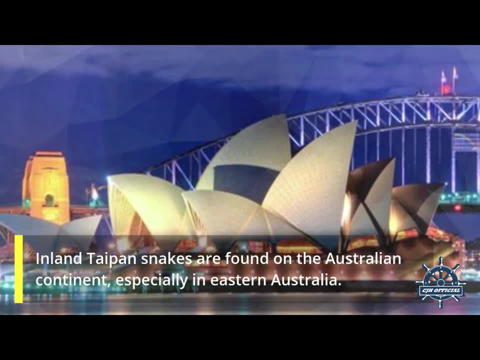 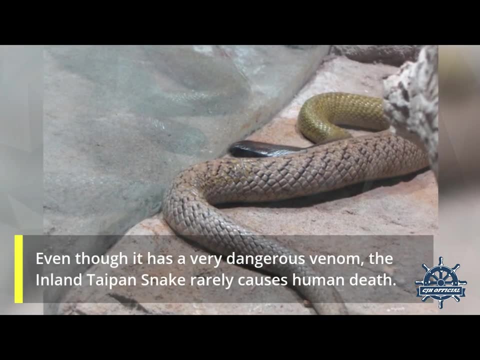 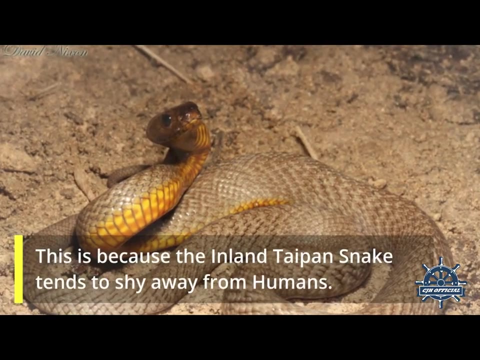 Inland Taipan snakes are found on the Australian continent, especially in eastern Australia. Even though it has a very dangerous venom, the Inland Taipan snake rarely causes human death. This is because the Inland Taipan snake tends to shy away from humans. 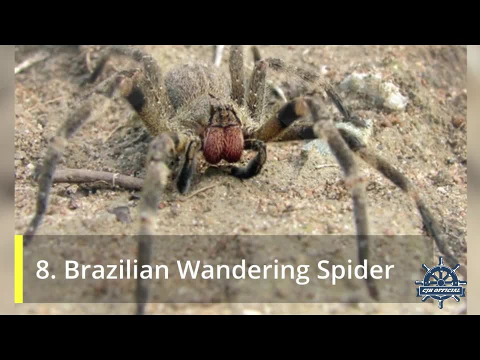 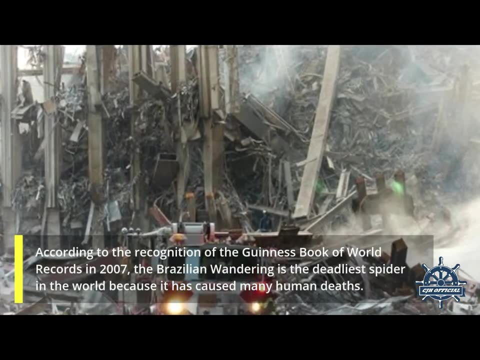 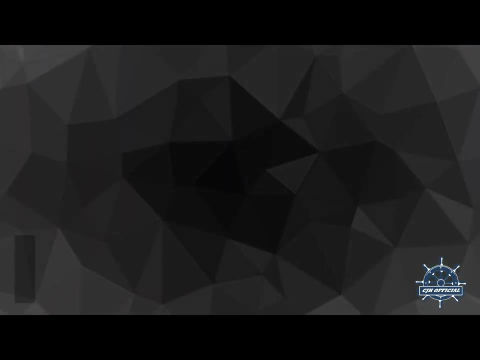 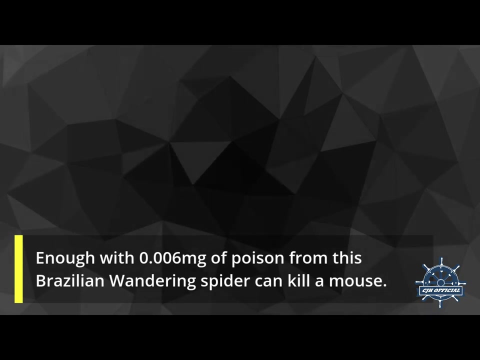 8. Brazilian Wandering Spider. According to the recognition of the Guinness Book of World Records in 2007,, the Brazilian Wandering is the deadliest spider in the world because it has caused many human deaths Enough. with 0.006 mg of poison from this Brazilian Wandering Spider can kill a mouse. 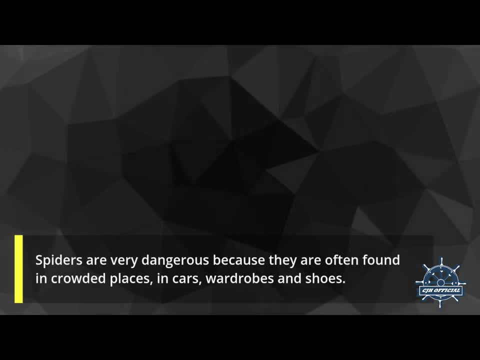 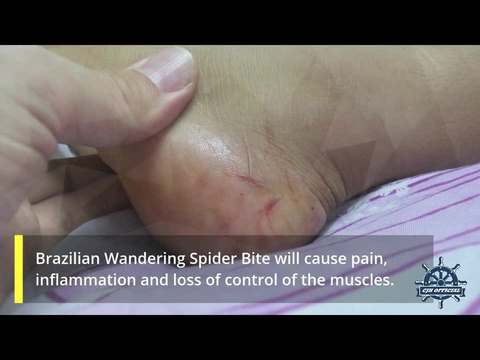 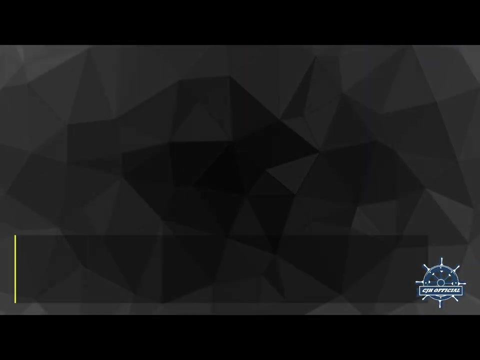 Spiders are very dangerous because they are often found in crowded places, in cars, wardrobes and shoes. Brazilian Wandering Spider bite will cause pain, inflammation and loss of control of the muscles. If not treated immediately, will cause death. Luckily, there is an antidote to this type of spider venom. 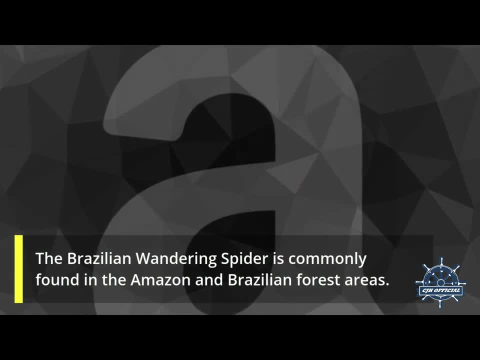 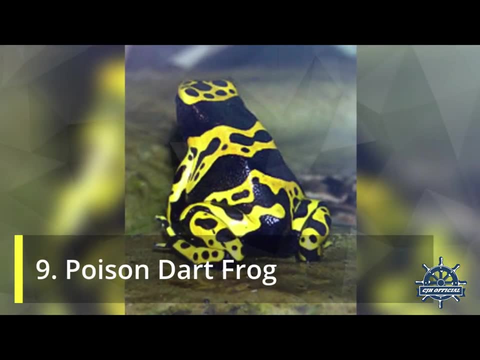 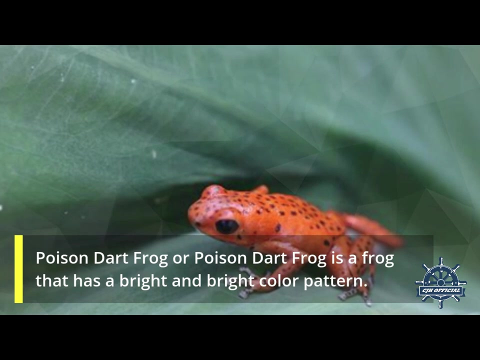 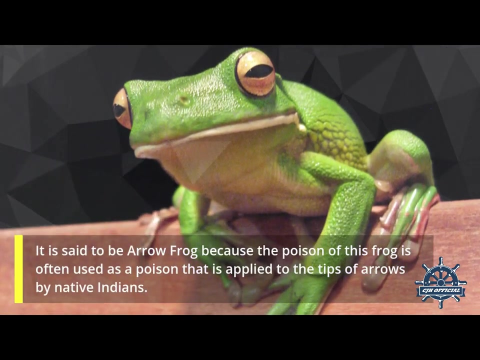 The Brazilian Wandering Spider is commonly found in the Amazon and Brazilian forest areas. 9. Poison Dart Frog. Poison Dart Frog or Poison Dart Frog, is a frog that has a bright and bright color pattern. It is said to be arrow frog, because the poison of this frog is often used as a poison that is applied to the tips of arrows by native Indians. 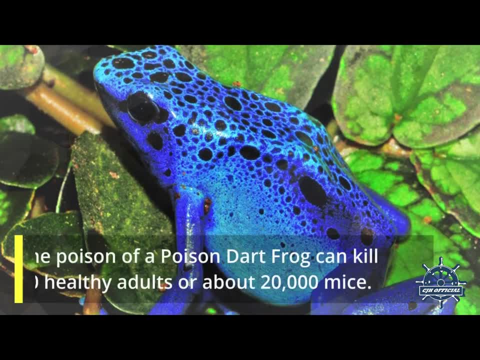 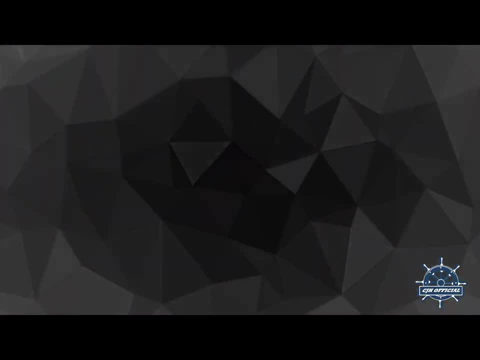 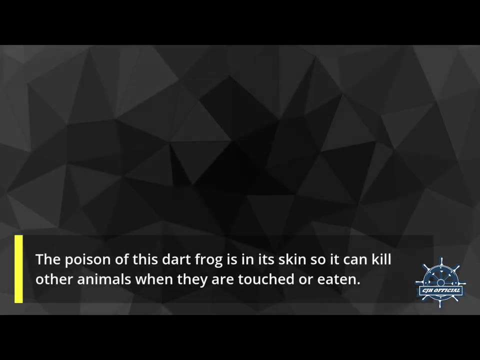 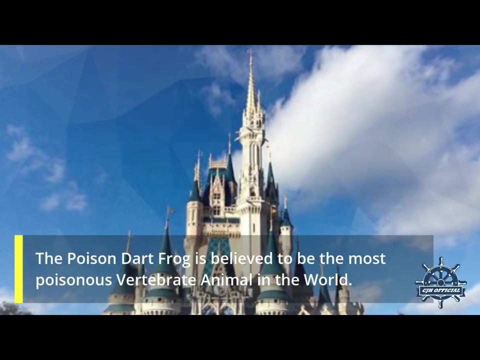 The poison of a Poison Dart Frog can kill 10 healthy adults or about 20,000 mice. The poison of this Dart Frog is in its skin, so it can kill other animals when they are touched or eaten. The Poison Dart Frog is believed to be the most poisonous vertebrate animal in the world.